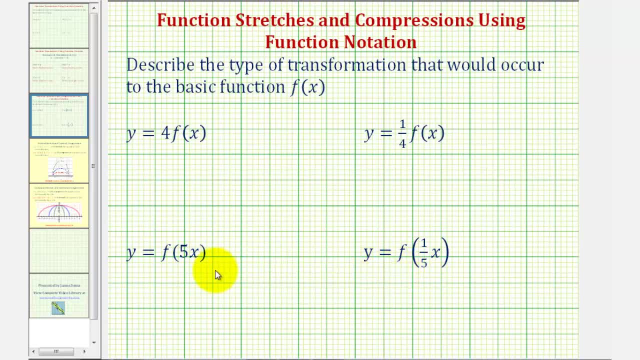 which will then affect the input of the function, And the inputs lie along the horizontal axis or x axis, and therefore, in this case, these two will give us either a horizontal stretch or a horizontal compression. To better understand what's happening here, let's take a look at some notes and some graphs. 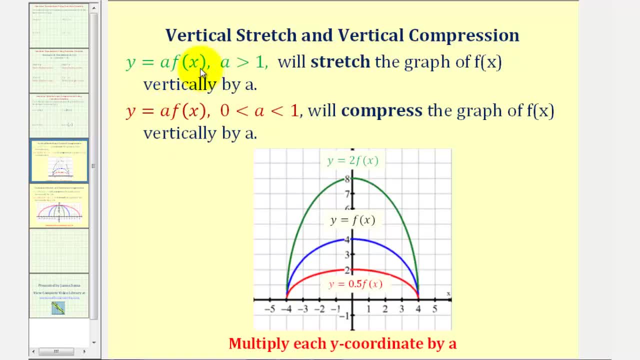 Let's first consider y equals a times f of x, where y equals f of x would be the graph of this middle. And if we look at the middle function here in blue, let's first consider what happens when a is greater than one. let's say a equals two. 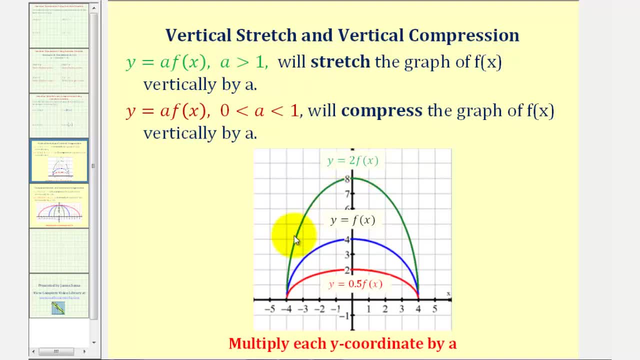 Notice, if we graph, y equals two times f of x, the graph is vertically stretched. The reason it's vertically stretched is because, in order to find the corresponding points on two times f of x, we multiply each y coordinate of the basic function f of x by a. 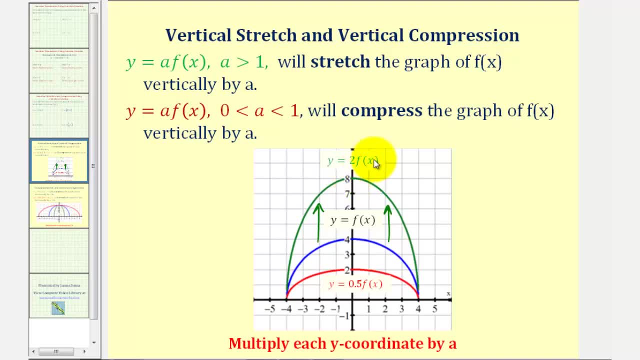 or in this case two. So because we're multiplying each y coordinate by two, we say this graph would be stretched vertically by two. Notice how the function values of f of x go from zero to four, but the function values of two times f of x go from zero to eight. 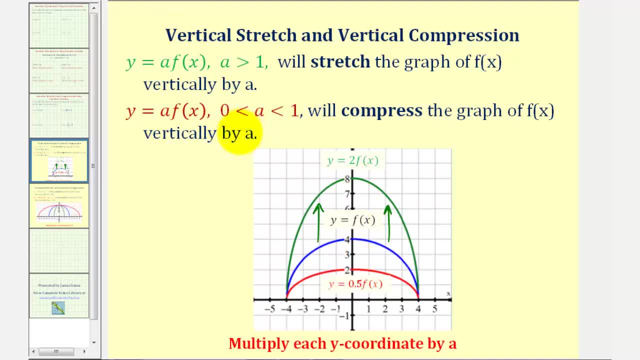 Now let's consider when a is between zero and one, or more specifically, let's say when a is 0.5 or one-half. Notice: the graph of y equals 0.5 times f of x is vertically compressed because to find corresponding points on 0.5 times f of x we would multiply each y coordinate. 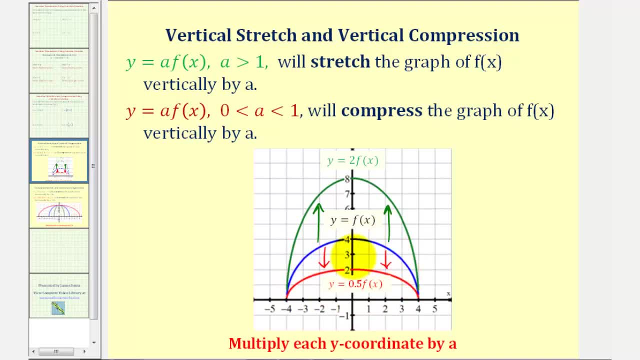 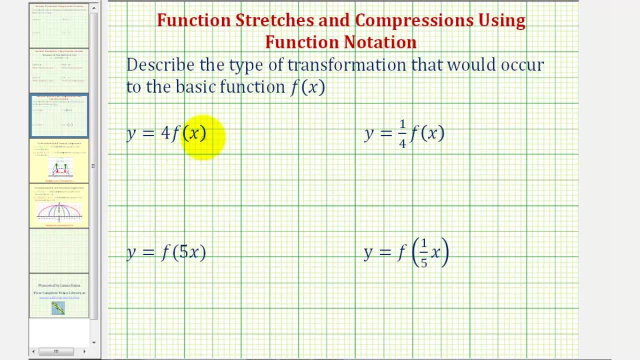 of the parent function f of x by one-half And therefore we can say: the graph of 0.5 times f of x would vertically compress f of x by one-half. So going back to our examples, if we have y equals four times f of x. 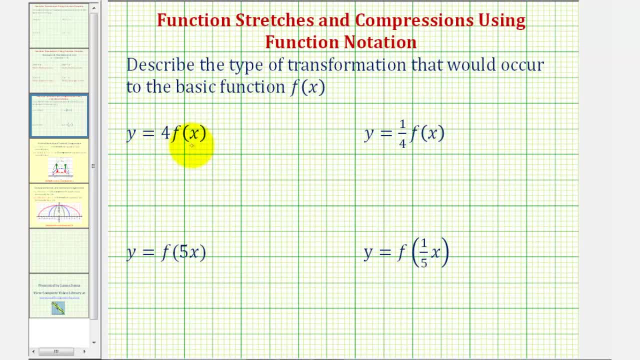 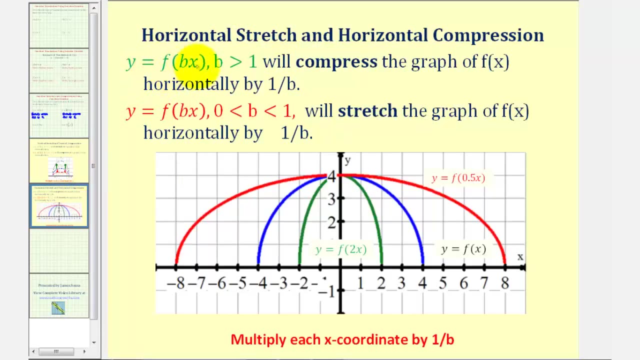 this will vertically stretch f of x by four. And for y equals one-fourth times f of x, this will vertically compress f of x by one-fourth. Now for these next two examples. let's consider y equals f of bx. Again, notice first: in blue we have the graph of the basic function: y equals f of x. 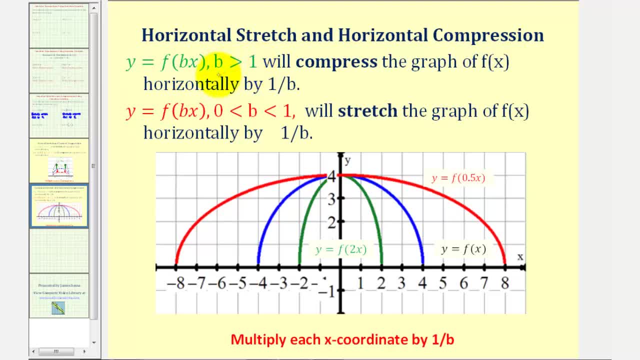 And now let's consider when b is greater than one. more specifically, let's say b equals two. Notice the graph of y equals f, of 2x is actually horizontally compressed. Notice, along the x-axis the parent function goes from negative 4 to positive 4,. 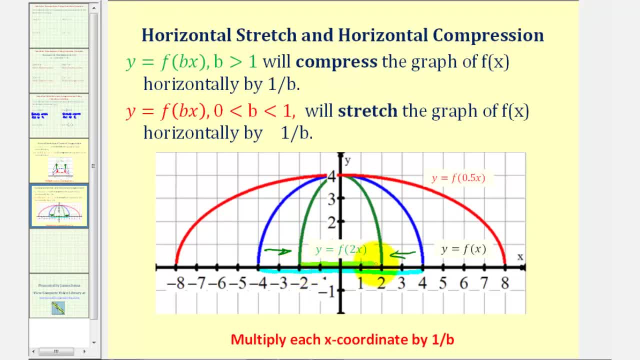 but f of 2x only goes from negative 2 to positive 2. So it's actually half as wide as the parent function. Let's talk about why that makes sense. Notice on the parent function. this point here and this point here would represent when f 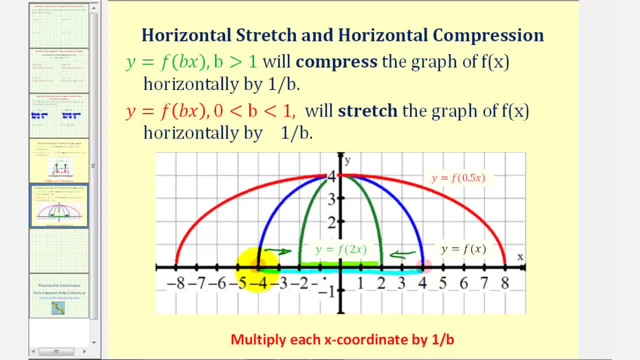 of 4 equals 0 and f of negative 4.. But notice on f of 2x, the input would be 4 and negative 4 when x is 2 and negative 2 because the input is 2 times x When x is 2. on f of 2x, notice that we would have f. 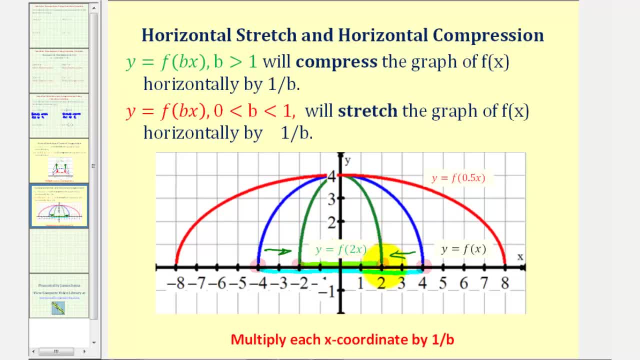 of 2 times 2, or f of 4,, which would give us the function value of 0., And when x is negative 2, the input would be 2 times negative 2, giving us an input of negative 4.. 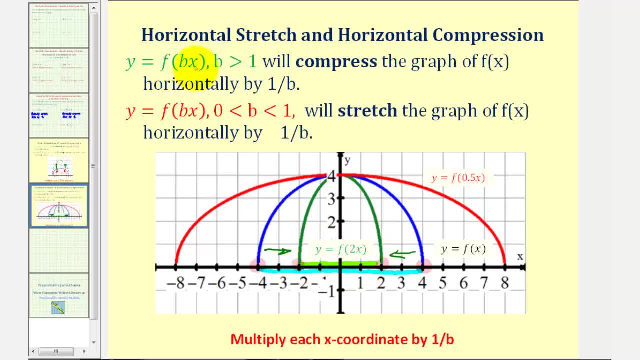 To find points on the function f of bx from the corresponding function. we have to find points on the function f of bx. To find points on the parent function f of x, we'd actually multiply each x-coordinate of f of x by 1 over b, not b. 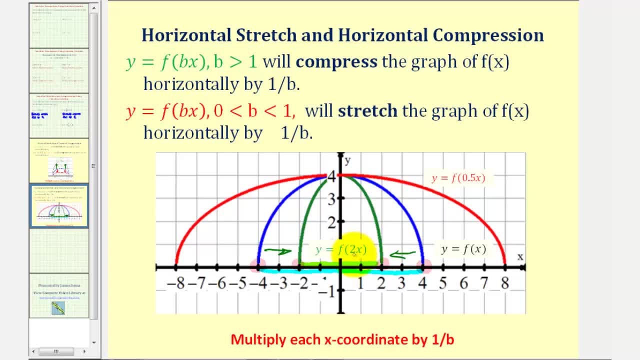 So in this case, notice how b is 2, so we'd multiply each x-coordinate on the parent function f of x by one-half, And because of this we say that when b is greater than 1, f of bx will compress the graph of f of x horizontally by 1 over b. 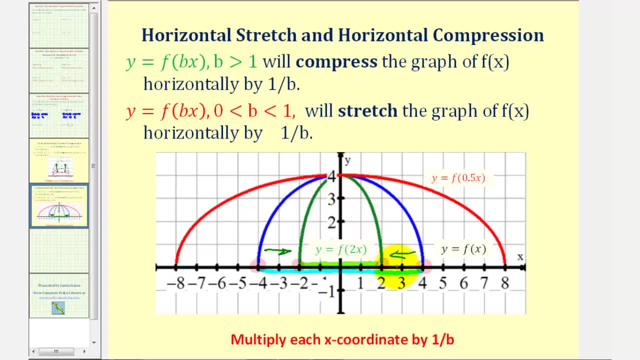 So the green graph is horizontally compressed by one-half, And when b is between 0 and negative 4, it will compress the graph of f of x horizontally by 1 over b. Notice how the red graph goes from negative 8 to positive 8 along the x-axis. 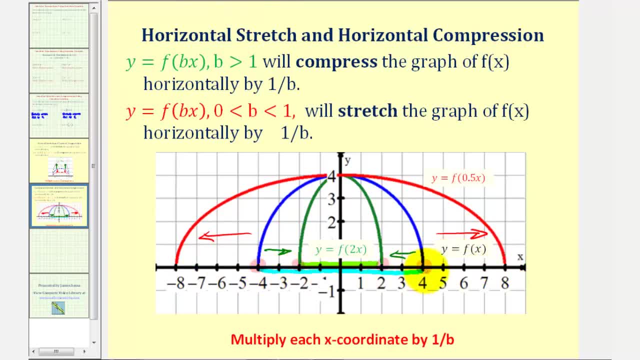 and their parent function only goes from negative 4 to positive 4.. The reason this should make sense again is because, notice, when x is 8 and negative 8, we would multiply these x values by one-half to determine the input into f of 0.5x.